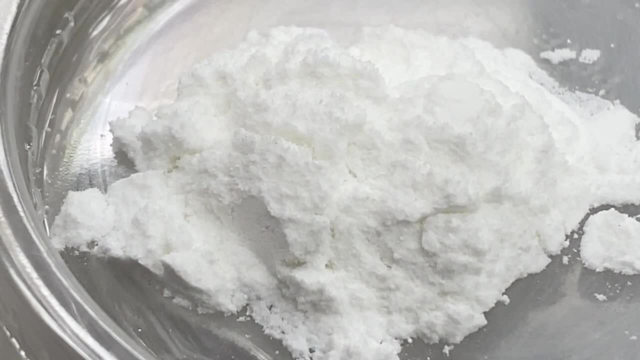 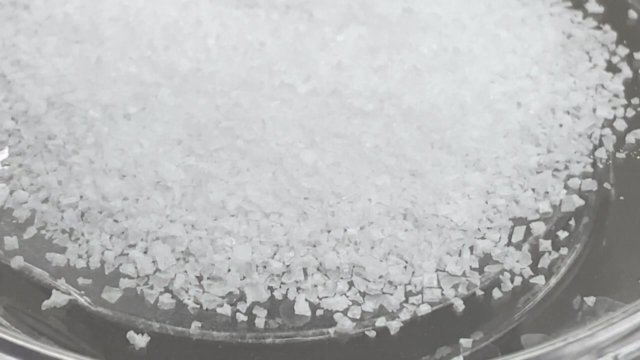 Diatomaceous earth is made up of shells of tiny aquatic organisms called diatoms. Diatomaceous earth is used in filters to remove heavy metals from water. Notice the color, the texture, the particle shapes and the particle size. This is kosher salt or sodium chloride, which is used to season food. 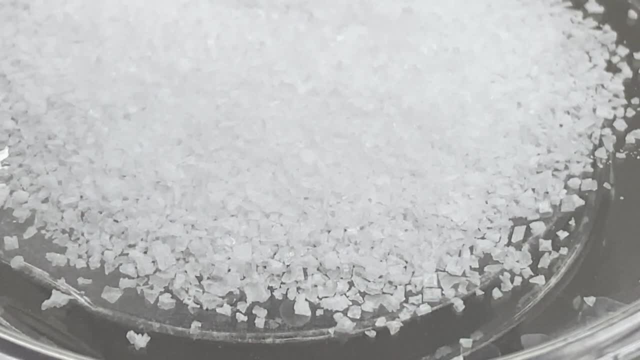 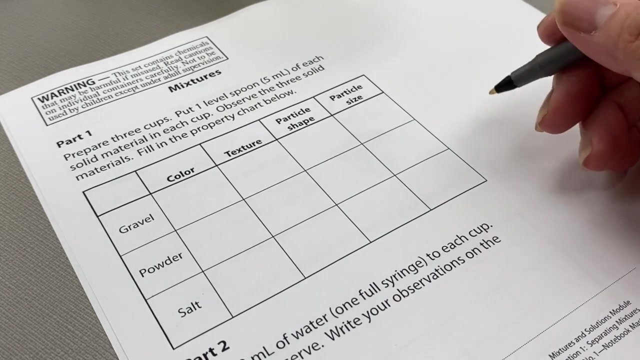 Notice the color, the texture, the particle shapes and the particle size. This is kosher salt or sodium chloride, which is used to season food. So how would you describe the color of the gravel? I saw black, brown and blue. I saw black, brown and blue. 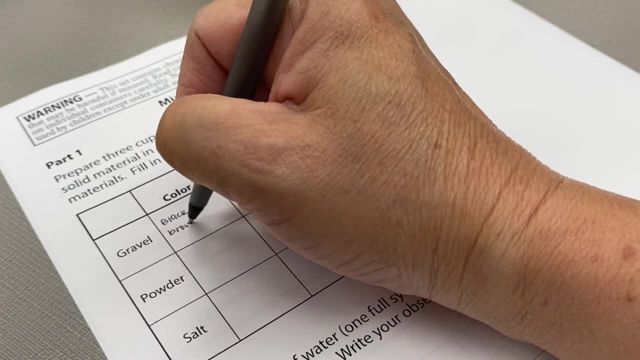 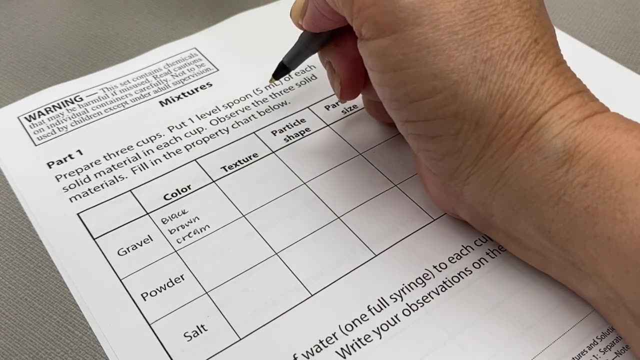 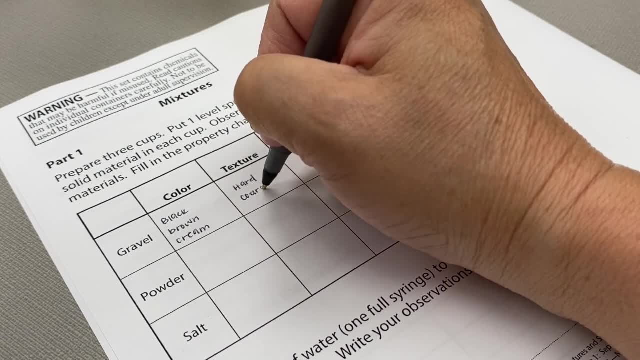 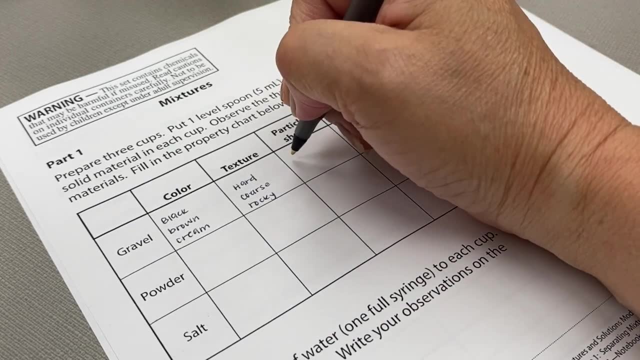 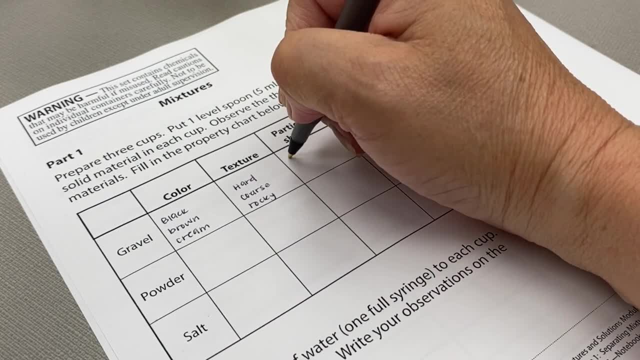 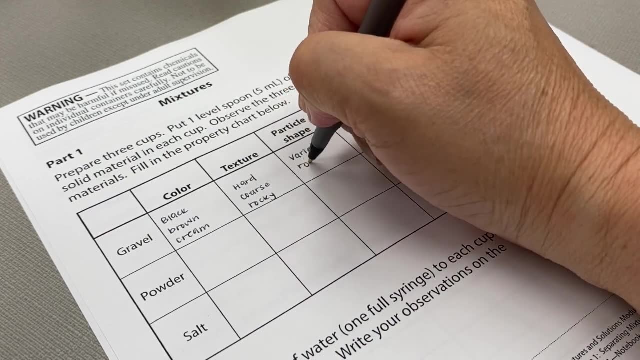 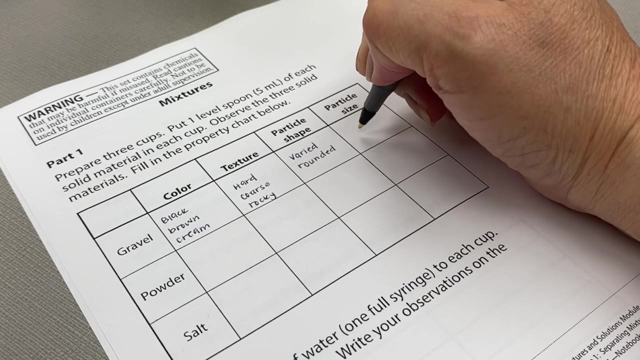 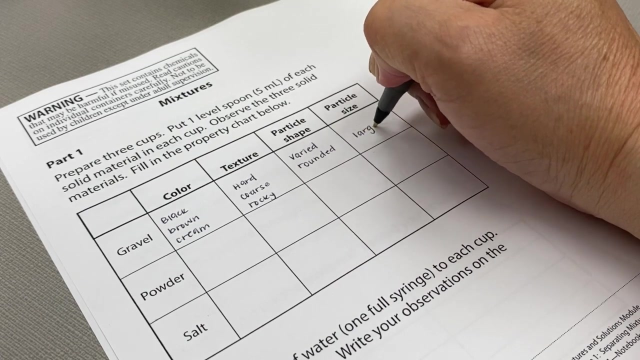 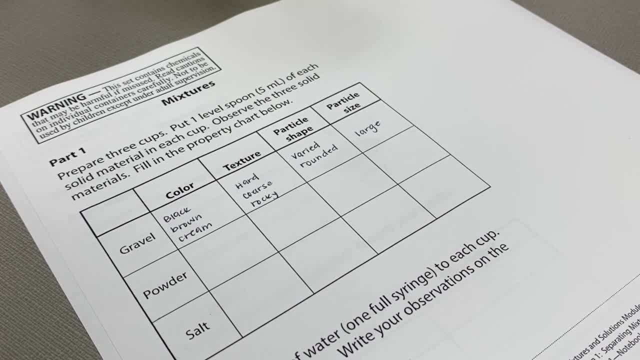 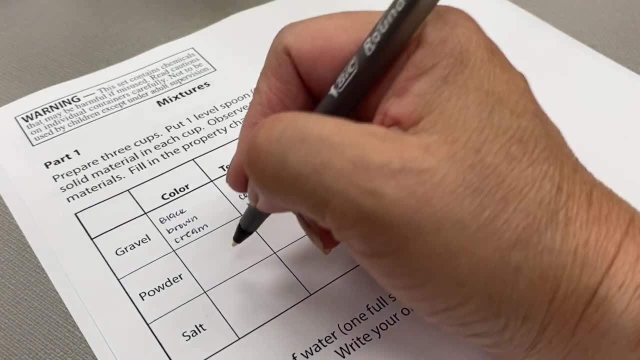 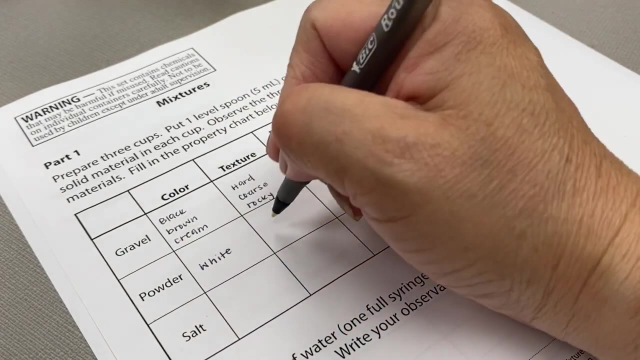 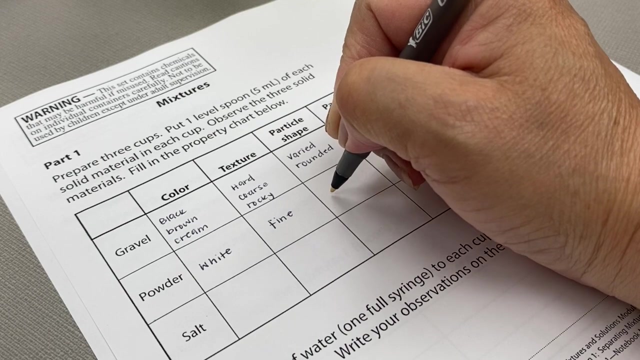 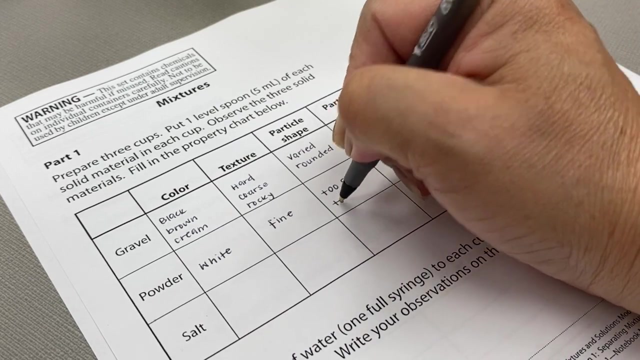 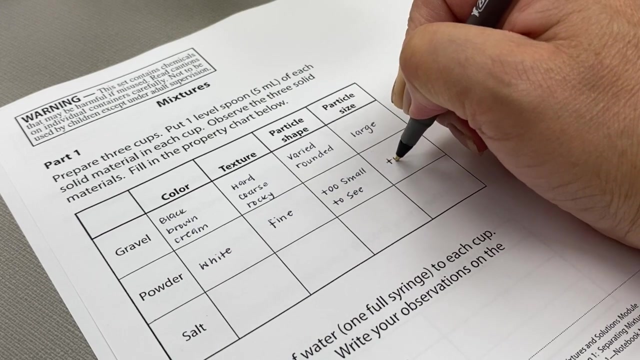 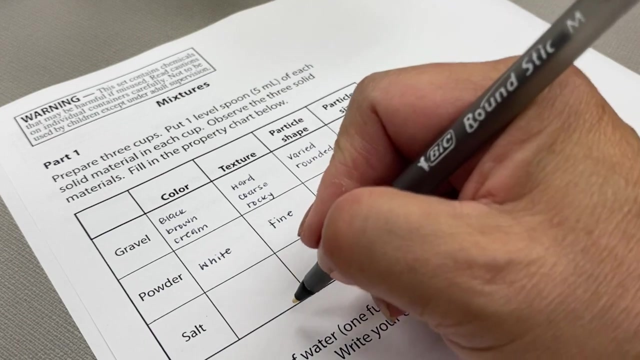 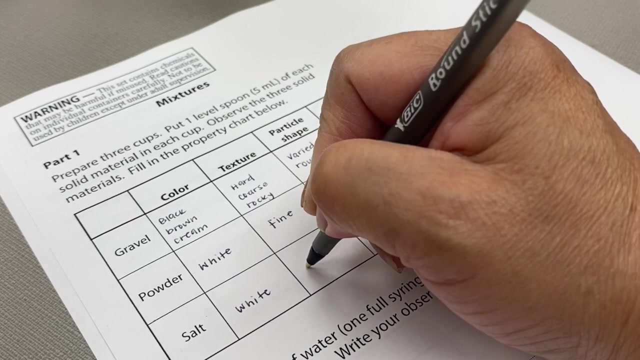 Next, let's look at our powder. What color was our powder? White Texture was fine. Particle shape: it was too small to see, Particle size tiny. Next, how about the salt? The color was white, The texture was coarse. 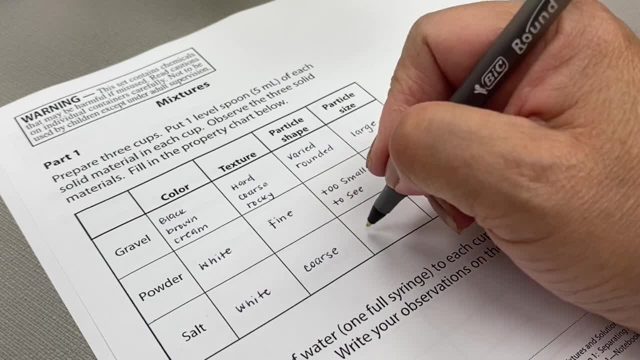 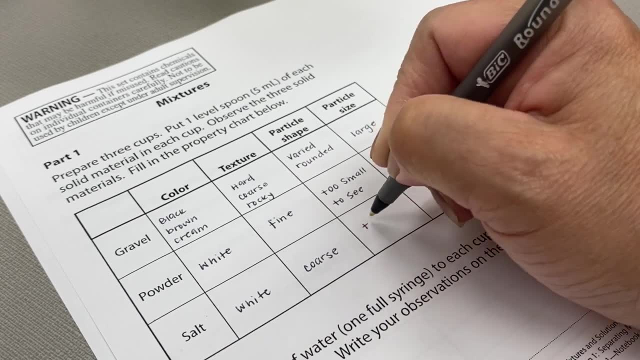 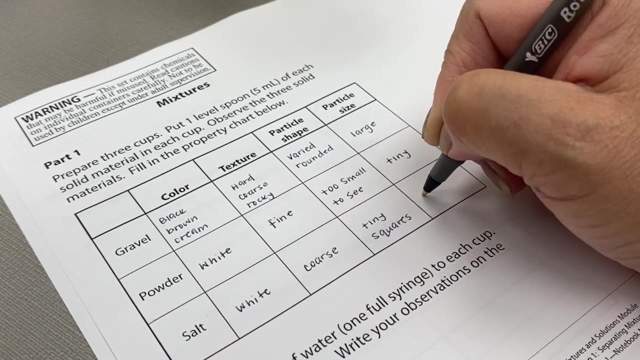 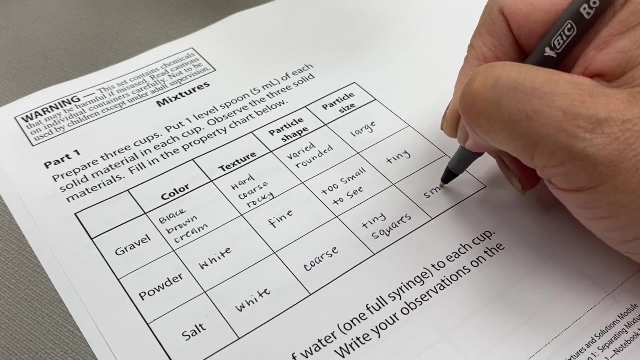 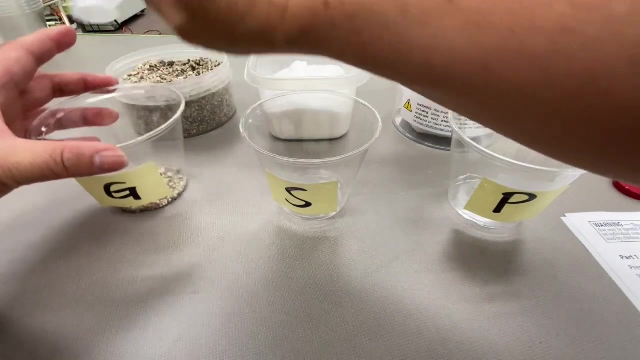 Not as fine as the powder. Particle shape: Almost tiny squares. And how about the particle size? Not as tiny as the powder and not as large as the gravel, but it was still small. Next, we will take one scoopful of each solid and put it in our cups. 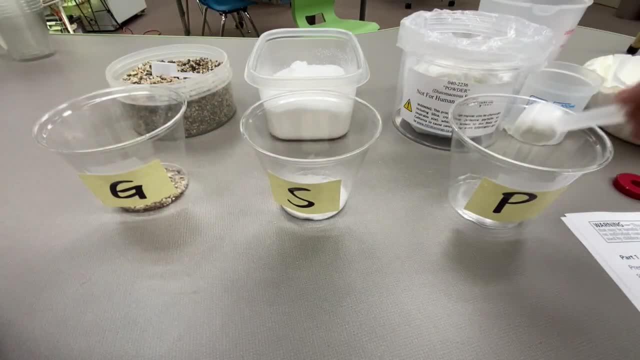 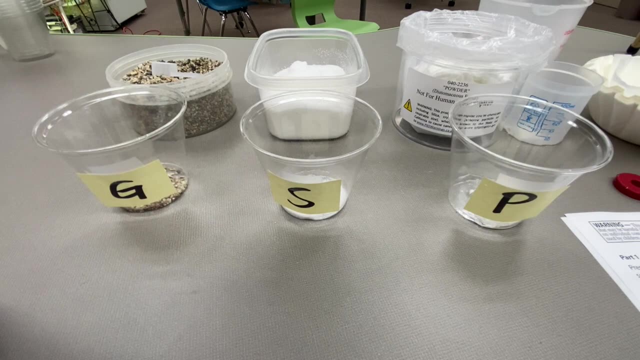 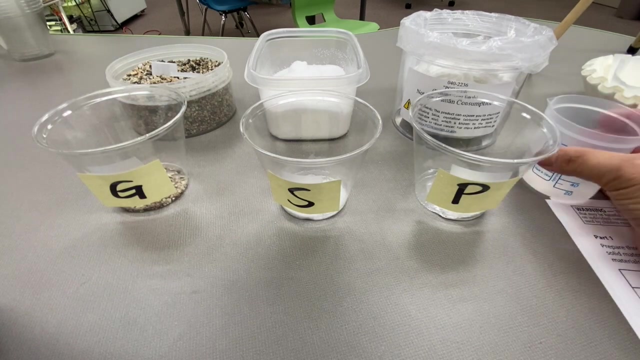 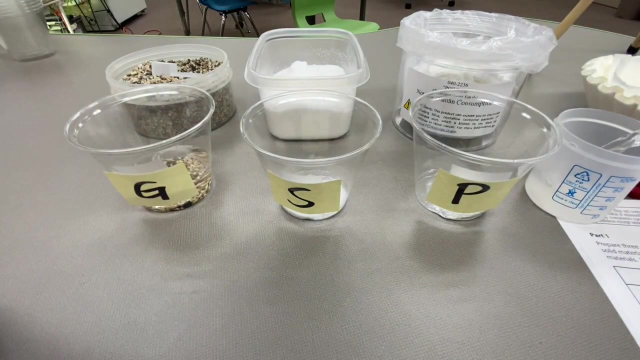 Okay, OK, so we get B, Let's go. What do you think will happen if I add water to each cup of dry materials? When you put two or more materials together, you make a mixture. If you like some different starchy and melty, you can add a little salt or a little bit of. 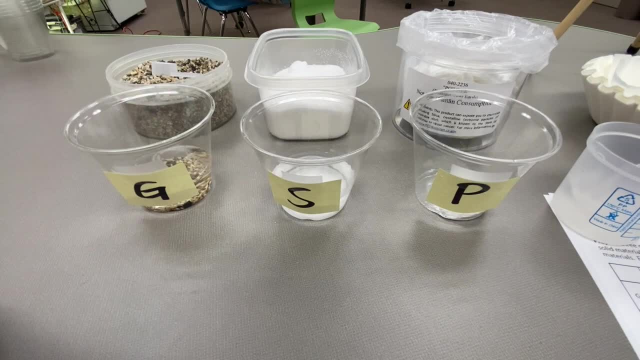 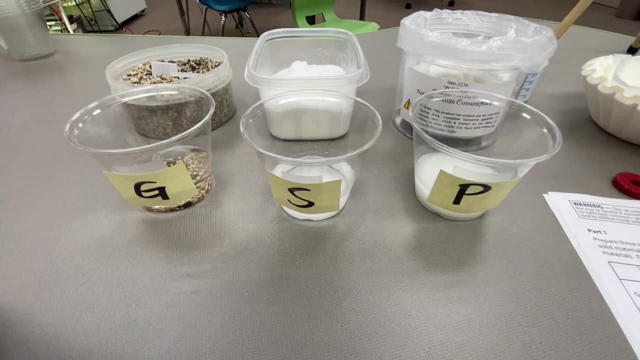 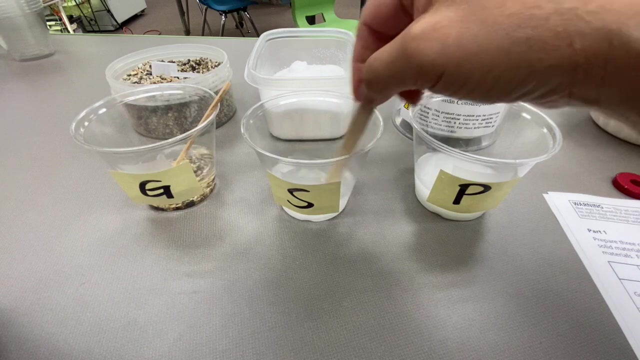 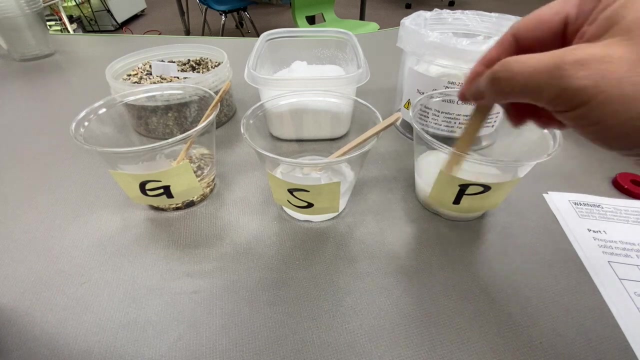 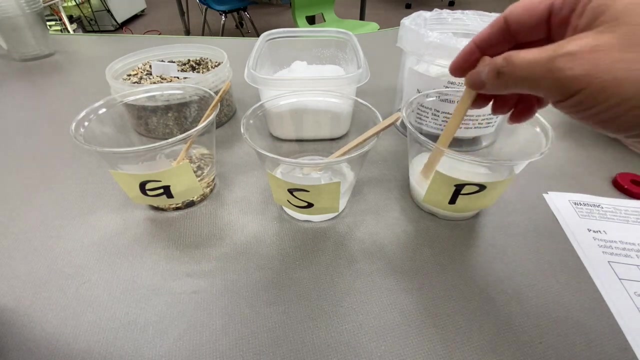 baking soda. But if you don't have baking soda, Go buenas, OK. So I have made three mixtures: gravel and water, salt and water and diatomaceous earth and water. We make mixtures at home all the time. 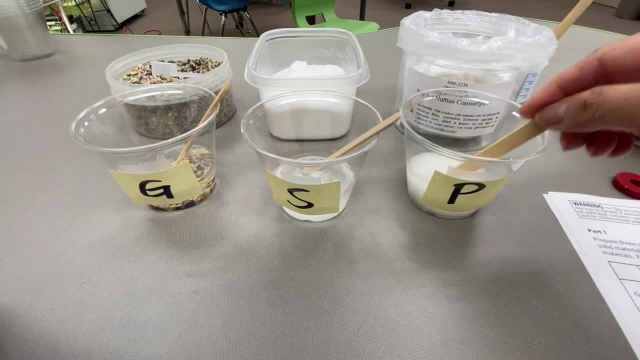 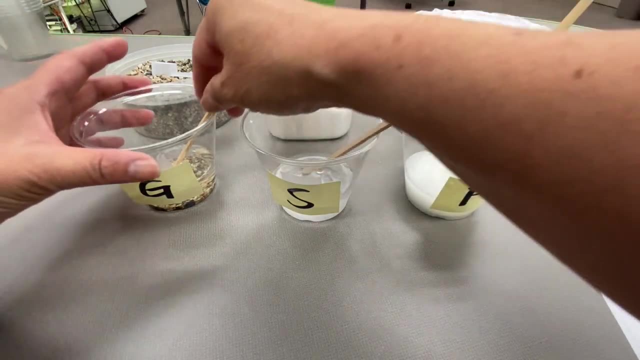 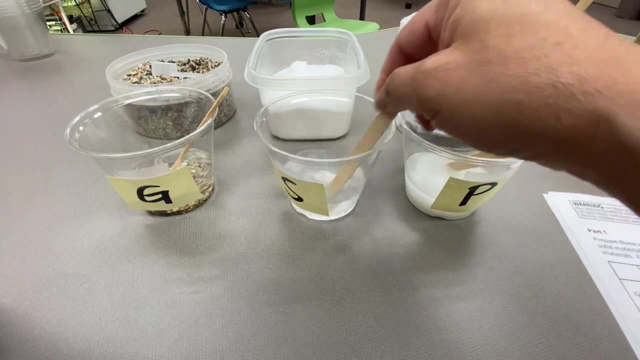 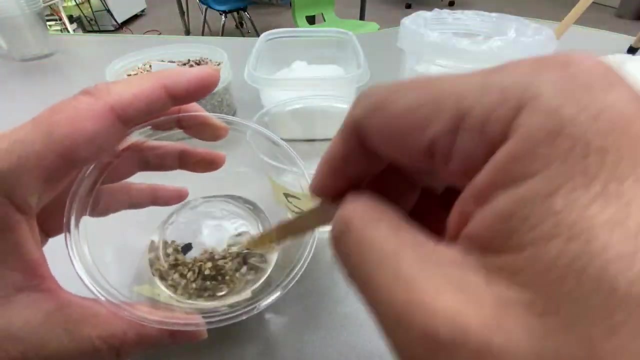 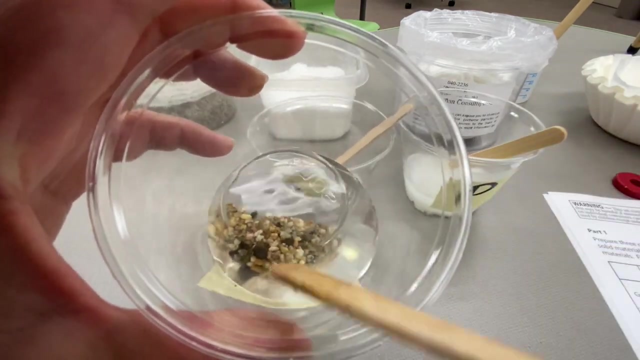 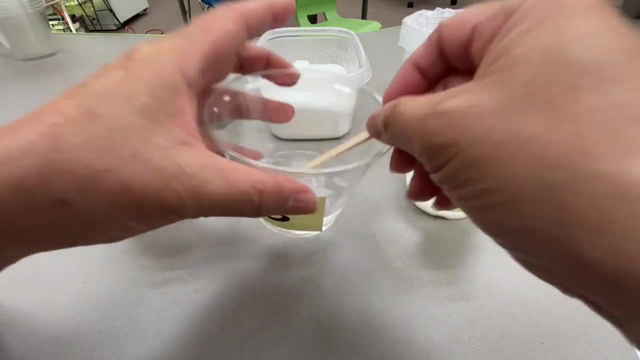 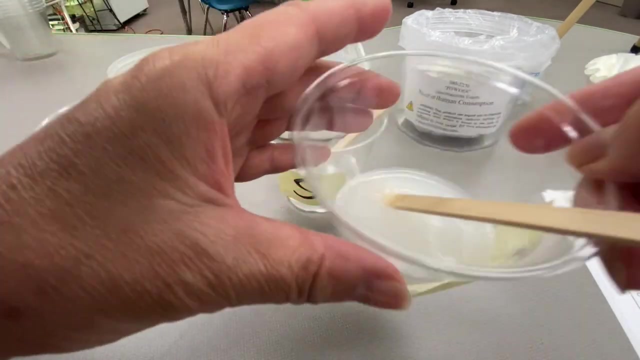 If you had cereal and milk this morning for breakfast, you made a mixture. If you liked chocolate milk, you made a mixture. So let's look at our mixtures. What do you observe happened in the mixture of gravel and water? What do you observe in the mixture of salt and water? 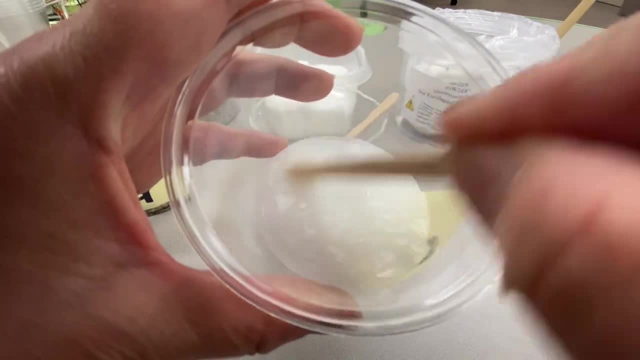 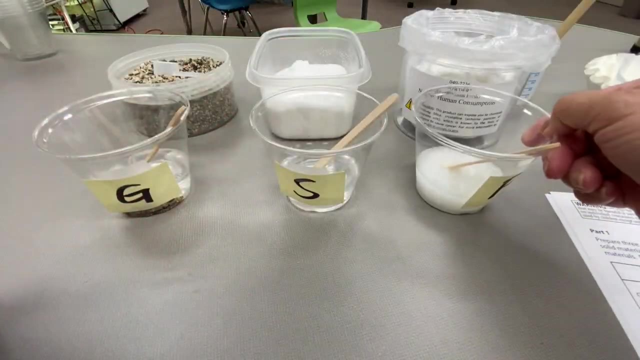 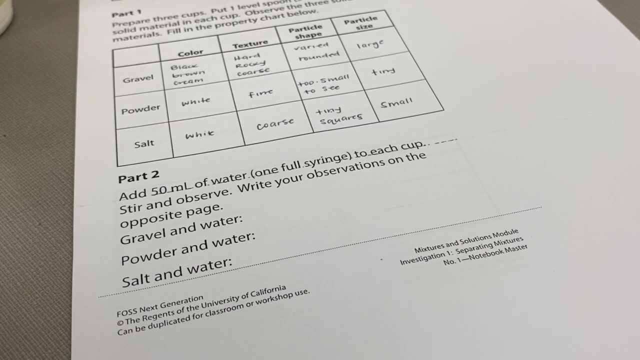 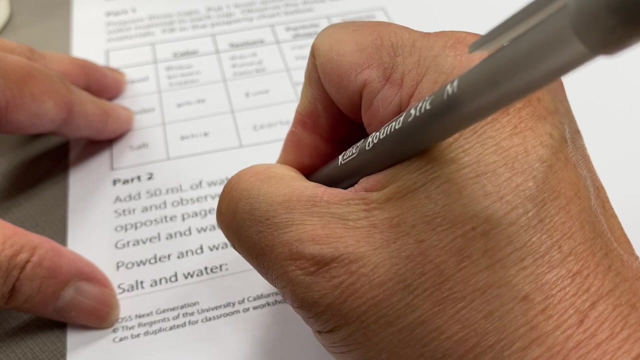 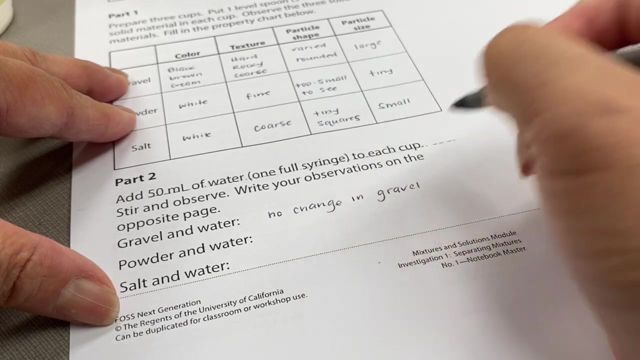 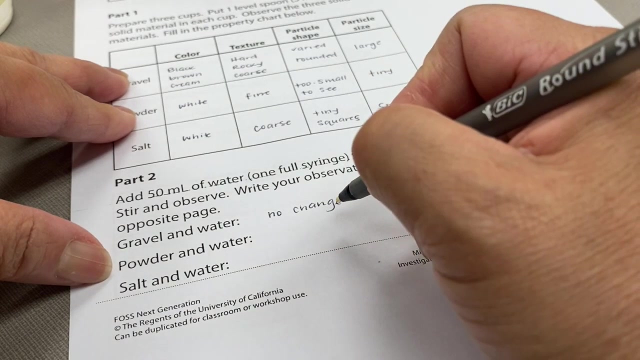 And what do you observe in the mixture of powder and water? Let's write down our observations on our data sheet. So what did you observe in our cup of gravel and water? No change in the gravel. How about the cup with powder and water? 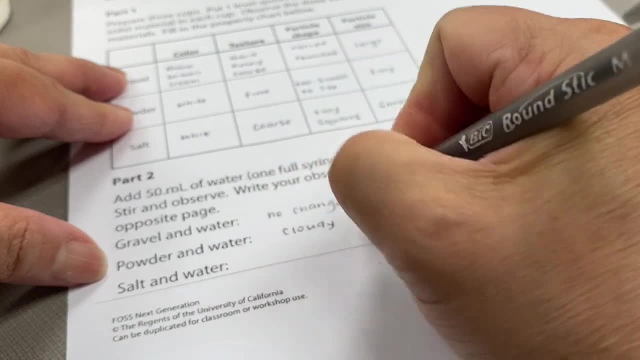 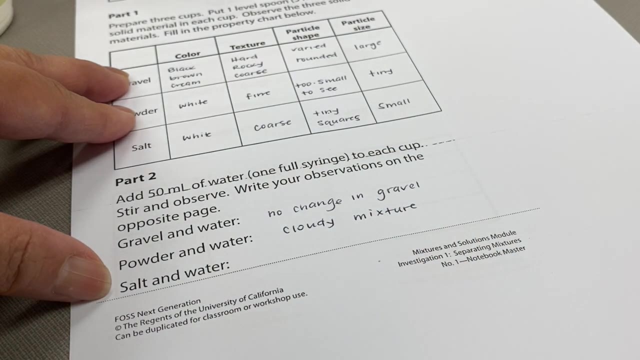 Cloudy mixture. Okay, Okay, Okay, Okay. So what did we observe? Love it picture. There it is. Lovely title. Let's add salt and water. Ooh, How about the mixture of salt and water? Salt disappeared. 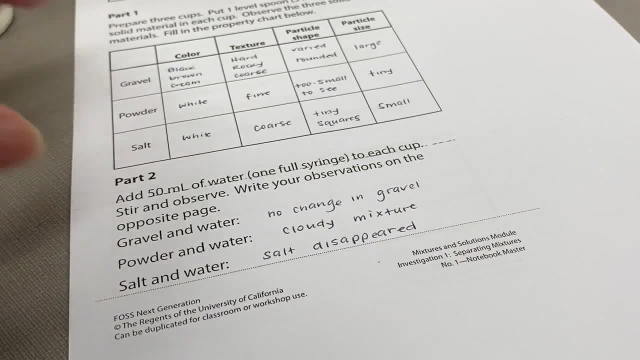 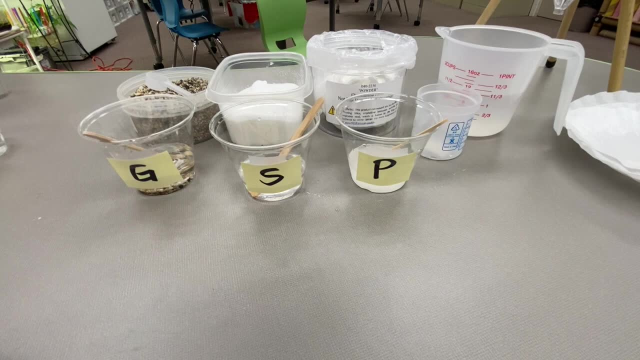 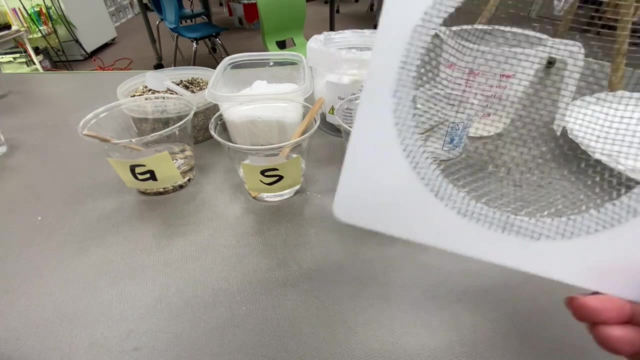 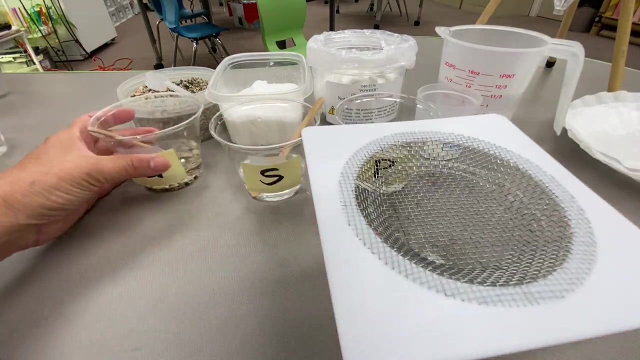 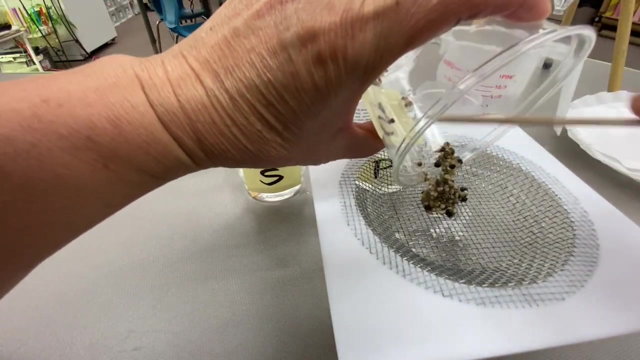 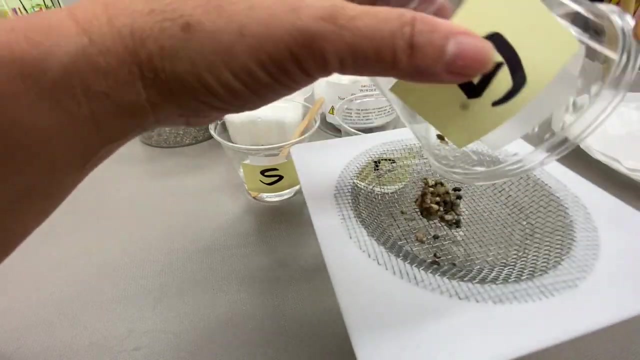 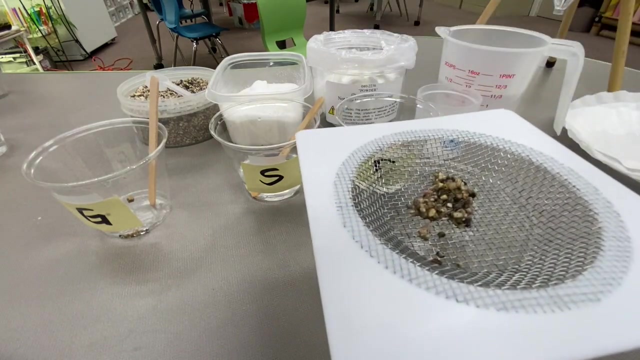 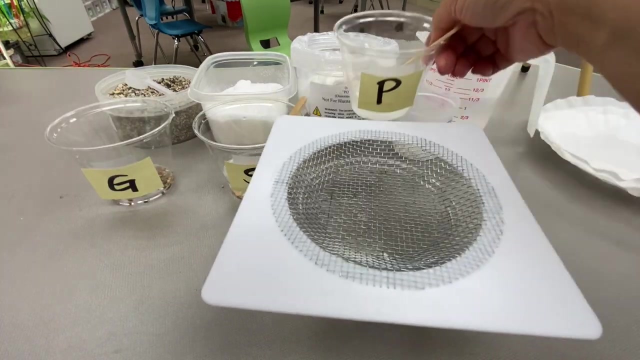 Now that we've made our mixtures, how can we separate them? Okay, Okay, Yes, a screen. Let's try separating our gravel mixture. That was successful from separating the gravel from the water. Next, let's try separating the water and the powder. 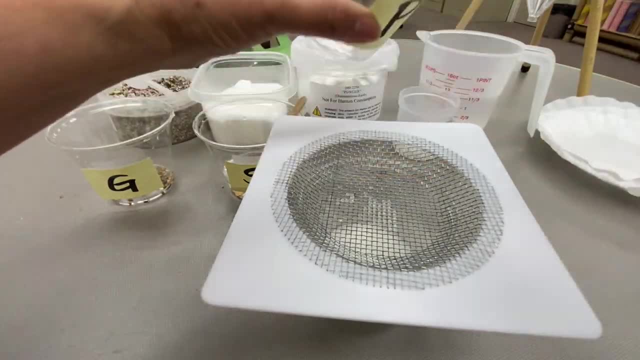 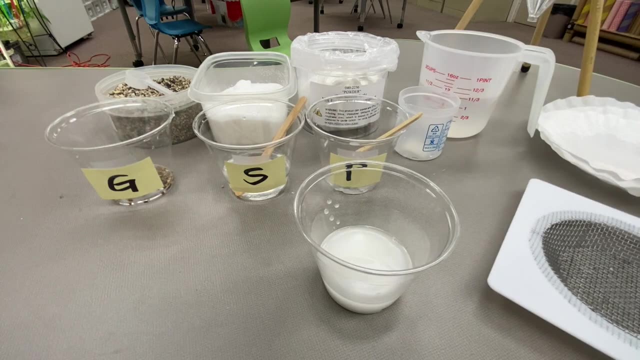 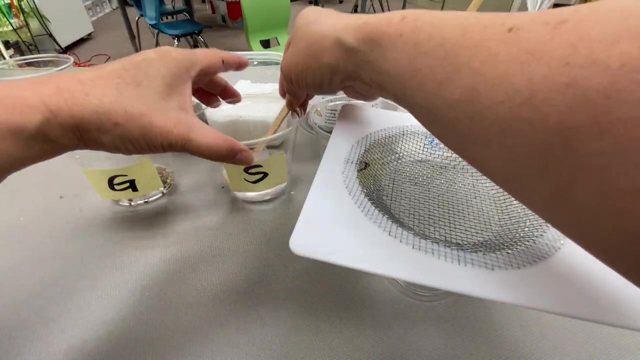 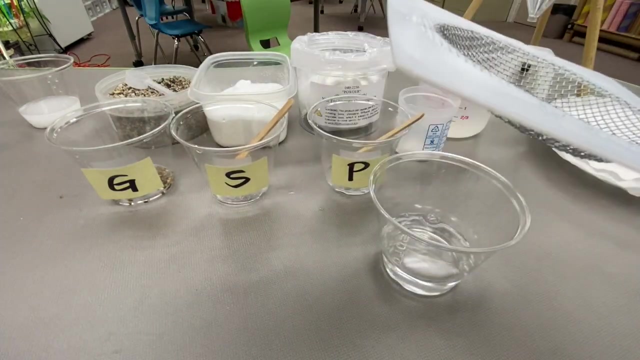 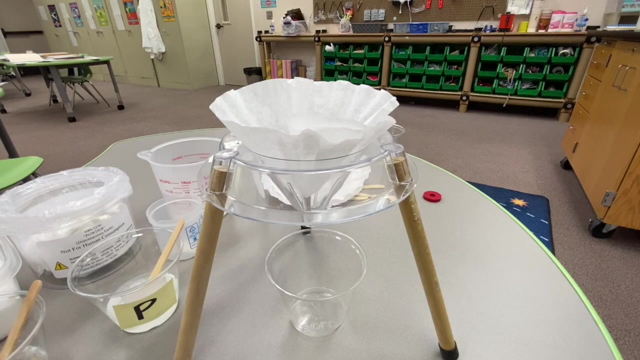 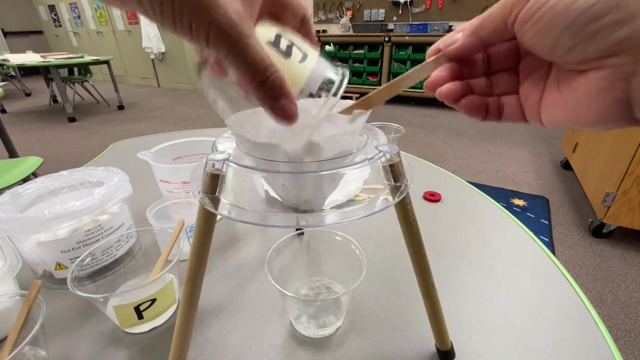 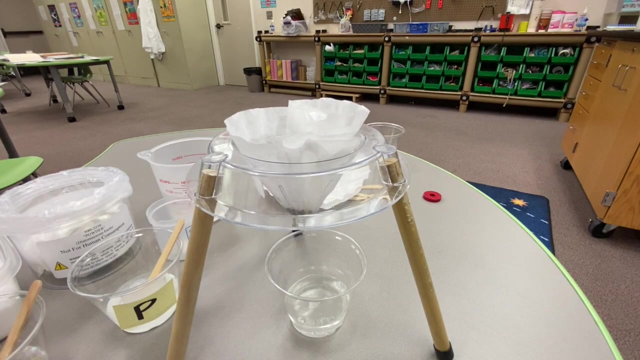 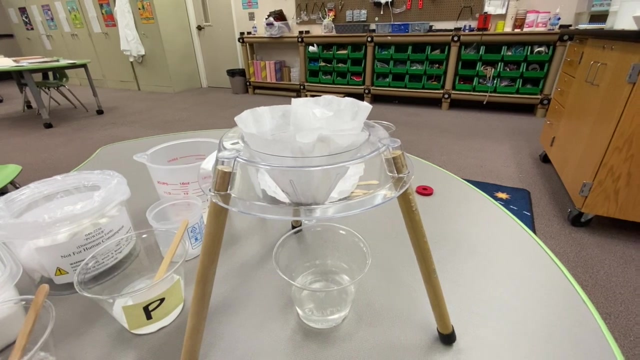 That was not successful in separating the water from the powder. Next, let's try separating the water and the salt. That, too was not successful in separating the water from the salt. Next, let's try using a funnel and a filter. That was successful in separating the gravel from the water. Next, let's try: 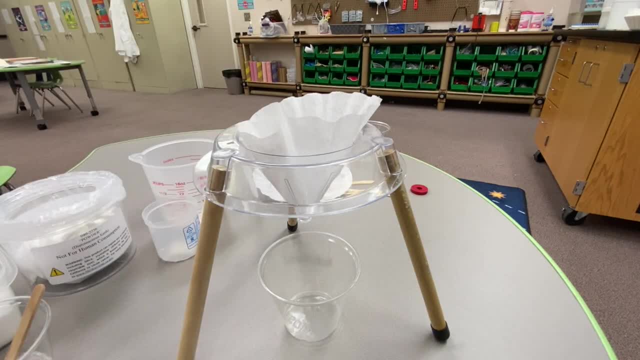 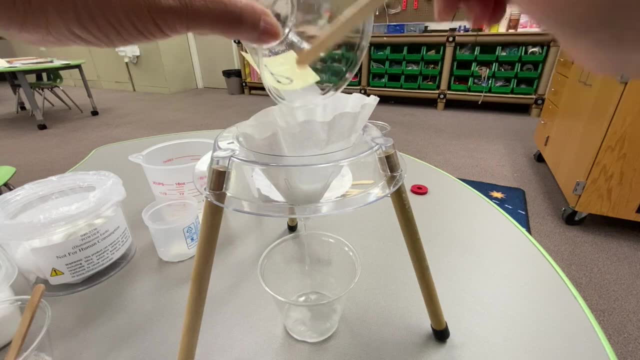 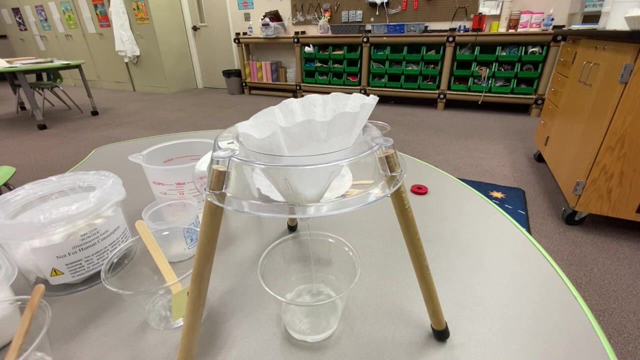 separating the powder and the salt. Let's try using a funnel and a filter. elujah, You can see that the cloudy water went in and only the clear water is coming out. You can see that the cloudy water went in and only the clear water is coming out. 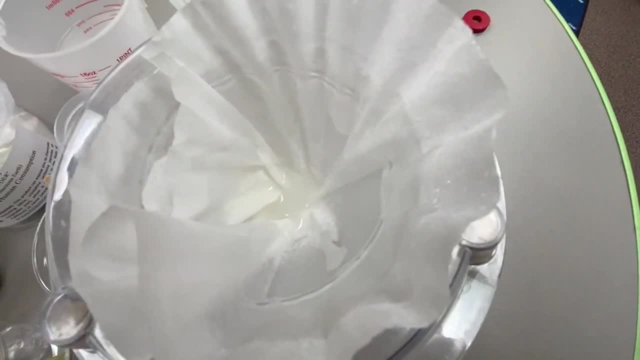 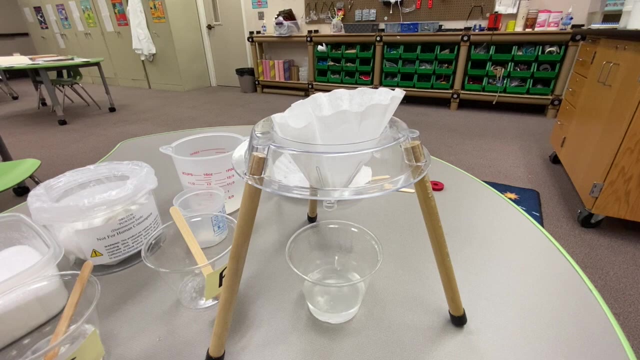 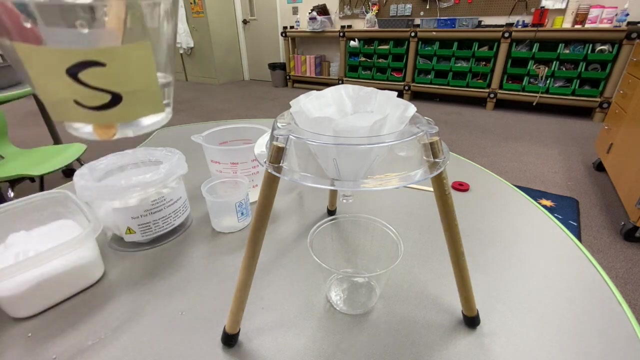 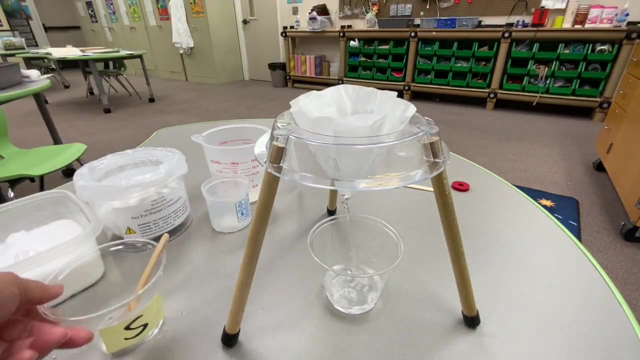 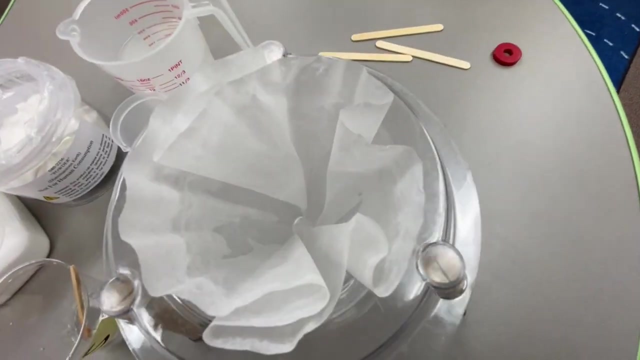 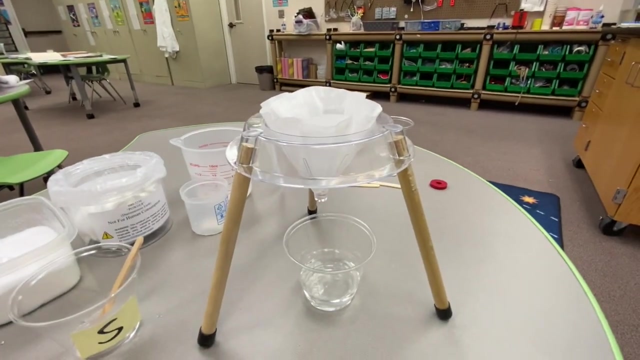 And you can see the powder collecting in the filter. So that was successful in separating our powder from the water. Next, let's try separating the salt from the water. There's nothing collected in the filter, so that was not successful in separating the salt from the water. 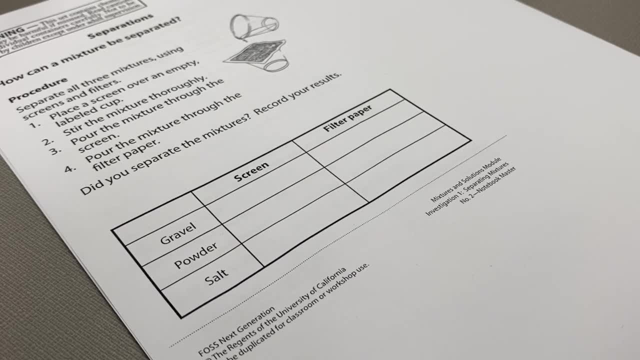 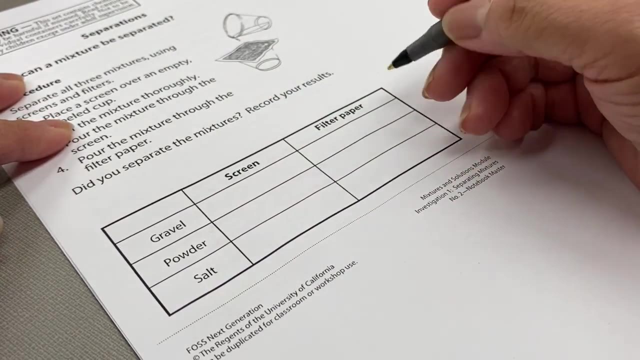 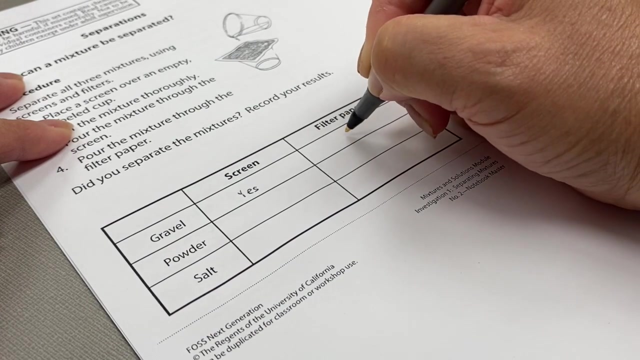 So let's look at our data sheet. What was successful in separating our mixtures For the gravel? was the screen successful in separating our mixture? Yes. Was the filter paper successful in separating our mixture? Yes, How about for the powder?